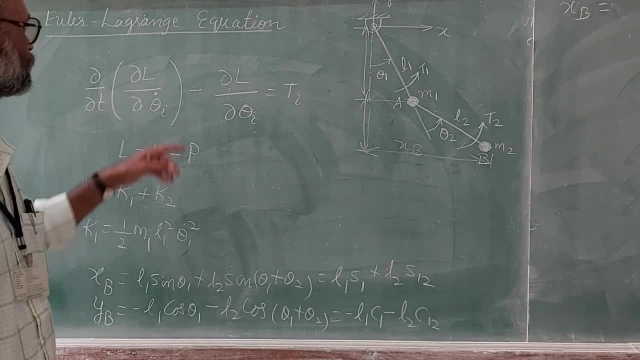 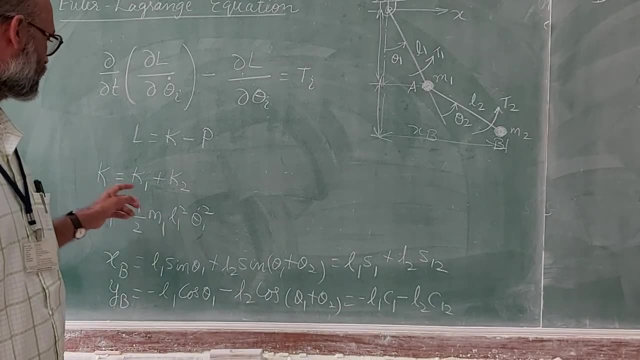 derive equations of motion for this problem. So first to derive Lagrangian for this equation. Lagrangian is given by kinetic inertia, So you have kinetic energy minus potential energy, Kinetic energy. if you look at this problem, kinetic energy, there are two masses, So you get two terms in kinetic energy. So 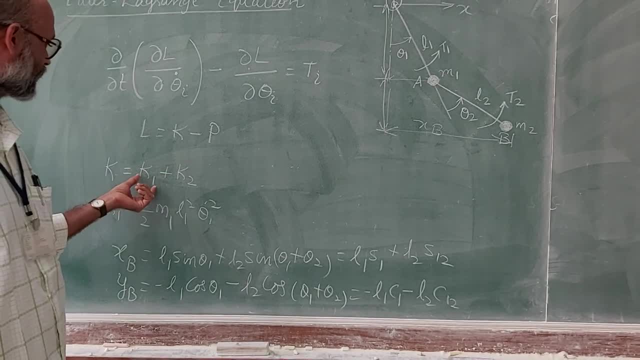 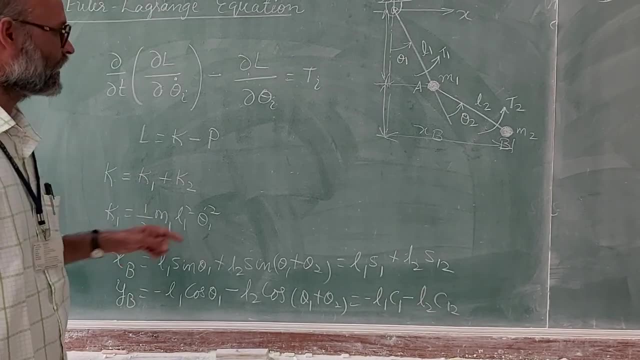 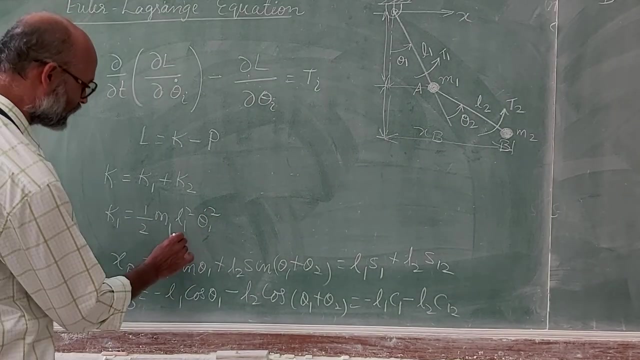 you have. kinetic energy of the total system is given by kinetic energy of the first mass and kinetic energy of the second mass, k1 plus k2, which is indicated there. And the kinetic energy of the first mass is given by half m1 l1 square, theta 1 dot square If. 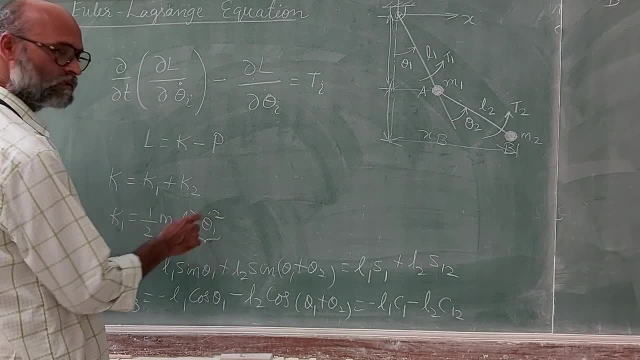 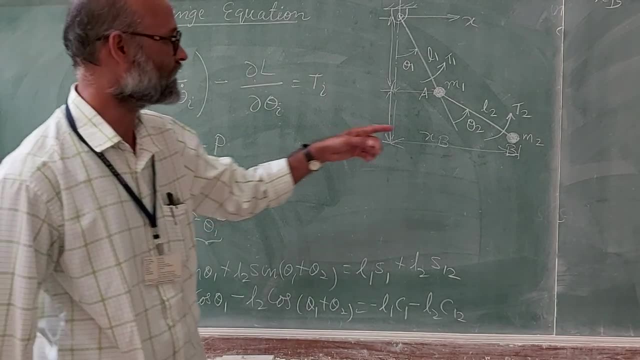 you look at this, this is your v square term: l1 square, theta 1 dot. So it is half m1 l1 square, theta 1 dot square. that is here To obtain kinetic energy for this mass m2, since it involves relative motion, we first figure out what is the position for. 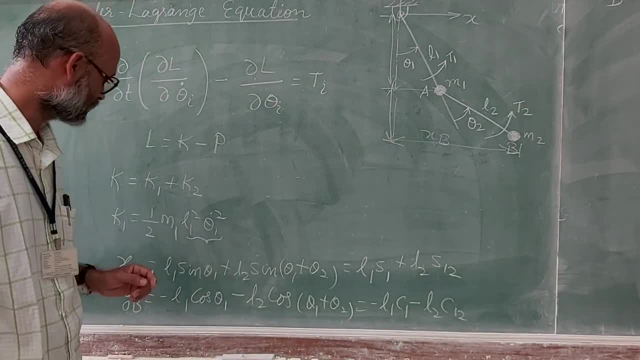 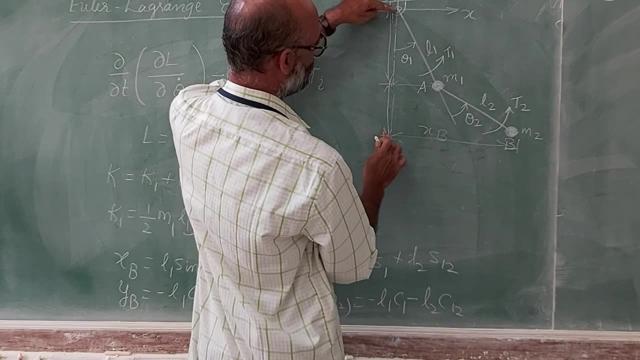 this mass, Then differentiate to get the velocity term for that. So what is the xv term? xv means from here. you can see: here, this is your xv and this part will be your yv term. This is yv from here to here, And this is here, this is here from here to here. So 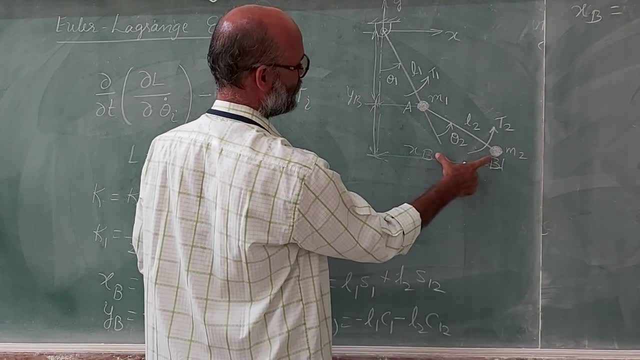 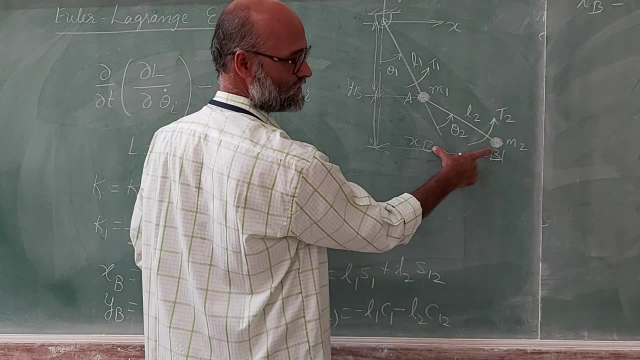 x d. If you figure out x d is this plus this much? What is this plus this one? This is l 1 sin theta 1, and this one is l 2 sin theta 1 plus theta 2.. That is what is indicated. 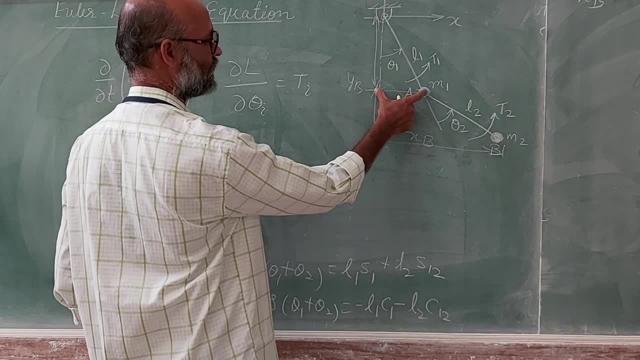 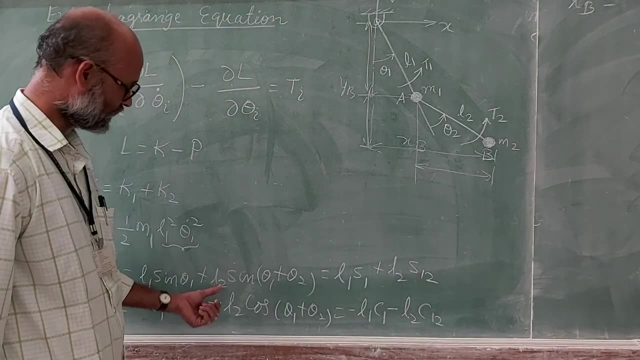 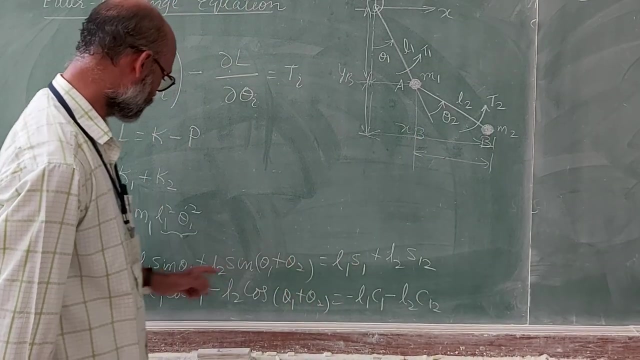 here l 1 sin theta 1. that is the term here. this plus this much Meaning. if you take this one, this distance, whatever you can see here, that is l 2 sin theta 1 plus theta 2.. This is l 2 sin theta 1 and theta 2.. In shortcut we will write theta 1 as sin, theta 1 as s. 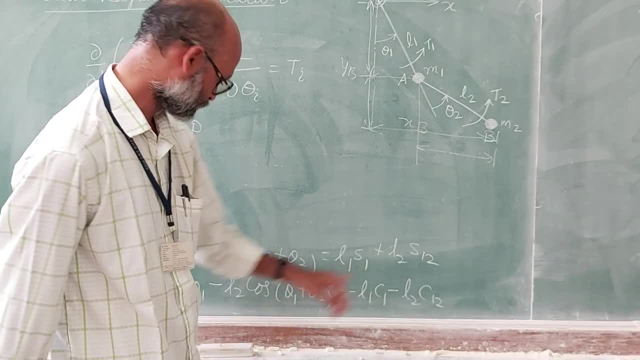 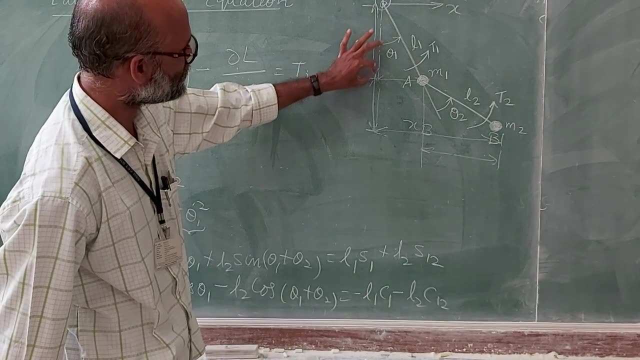 1 and sin theta 1 plus theta 2 as s 1, 2.. So that is the notation we follow all through this chapter. What about y p, y p? is this plus this term? So this term is l 1 cos theta. 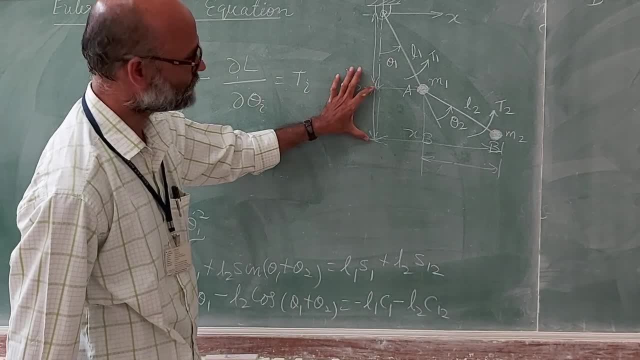 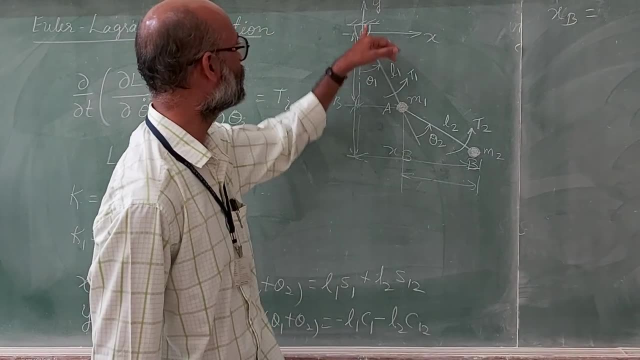 1. that is what I have written here, And this is l 2 cos theta 1 plus theta 2.. In shortcut it is written as l 1 c 1 minus l 2 c 1. This is negative because plus y is above, minus y is below, So x d is l 1 s 1 plus l. 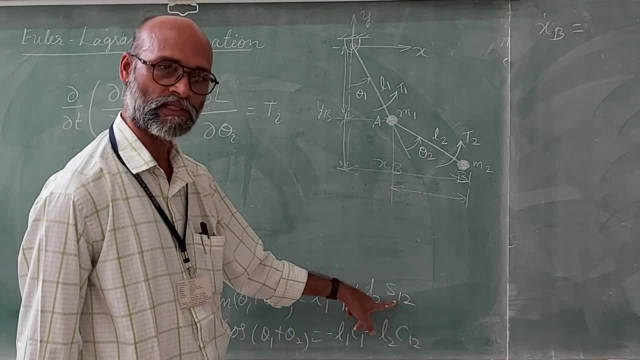 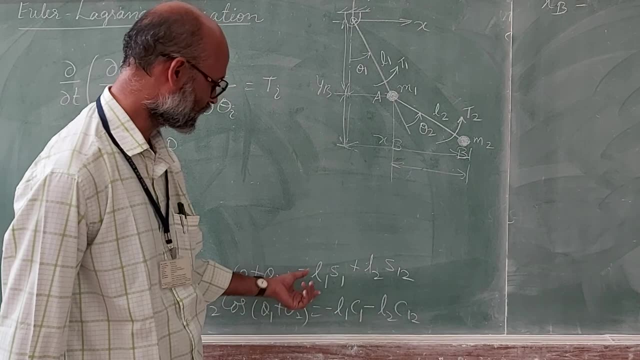 2, s 2. I repeat: s 1 is sin theta 1.. s 1: 2 is sin theta 1 plus theta 2.. c 1 is cos theta 1.. c 1: 2 means it is cos theta 1 plus theta 2.. Please ensure the notations you understand. 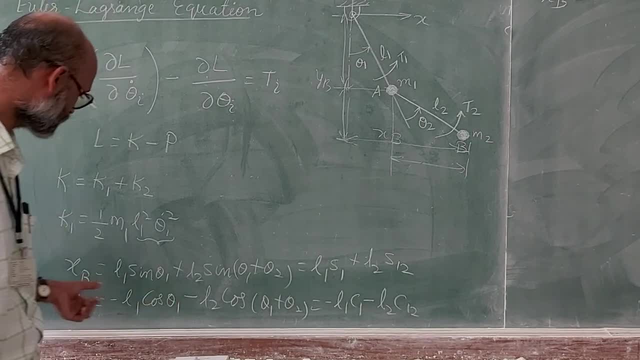 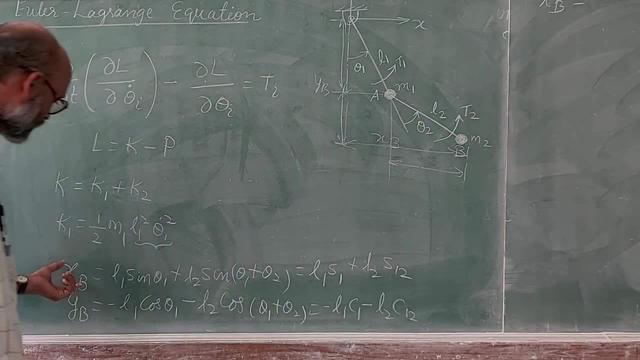 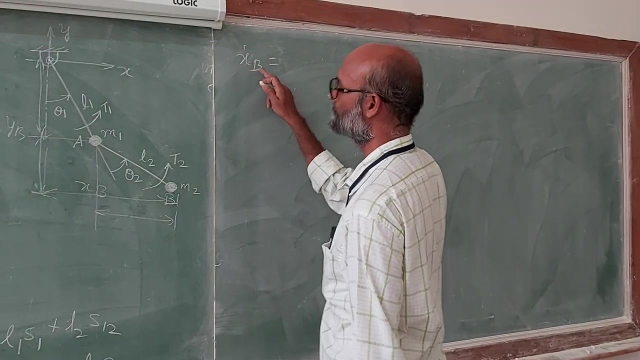 correctly, So that further calculation becomes easy. So this is the position for this big mass, m 2, which I have termed it as v. So we will differentiate this x d and y d and then get the equation for velocity. When you differentiate x d, what do you order the coefficient here? You can see here: l 1, c, 1. 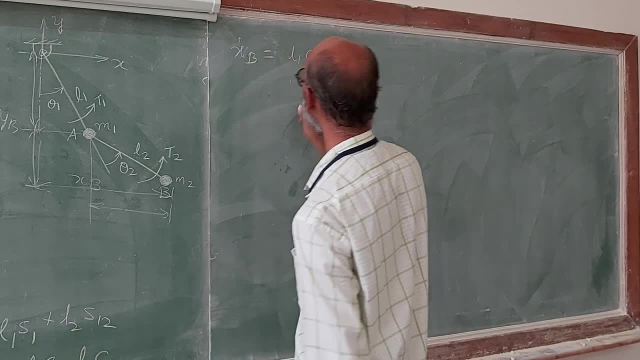 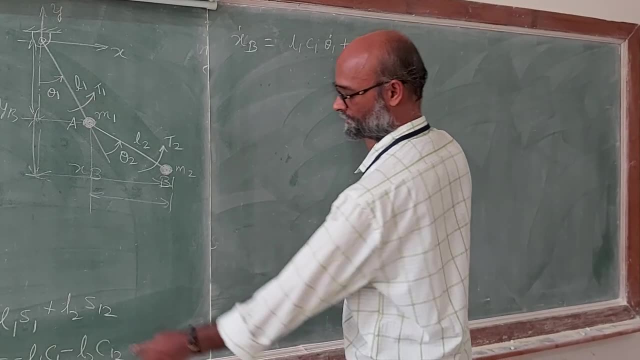 theta 1 dot. So when you differentiate l 1 s 1, this is l 1 c 1. differentiation of sin theta is cos theta and theta 1 dot. And plus differentiation of this is l 2 c 1, 2 this. 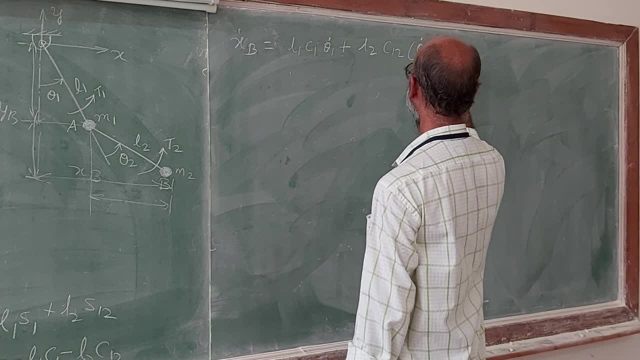 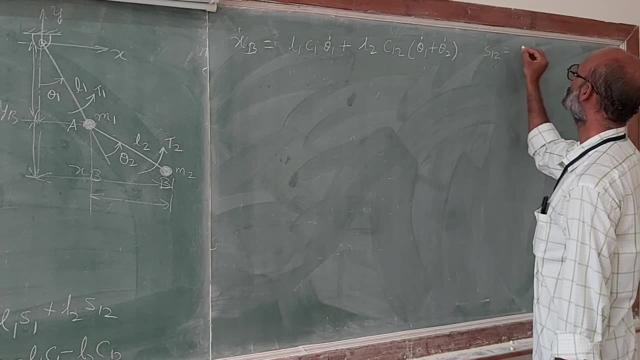 will come as theta 1, dot plus theta 2.. So this is the equation for velocity. So we will consider theùf flrain velocity for velocity here. So now we are going to think about the l 2 yet to l 1igrade of v. Now the function of velocity of v here happens to be G minus. 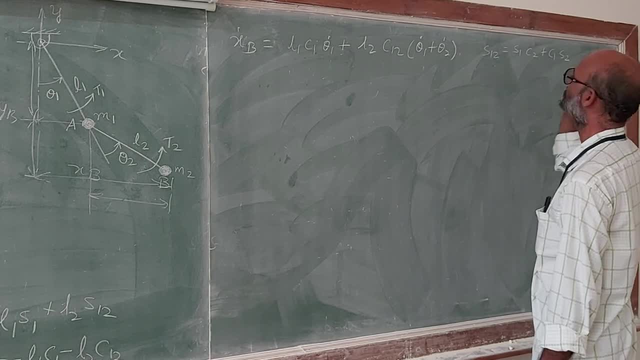 1. The faster it goes, time side function, The faster the velocity is a Sty he power velocity. So we are try to choose the vector r by b, So anytime it is running over the coś which is h1, v z dot v or we are still decrease the game because w 2 devices, Oops. 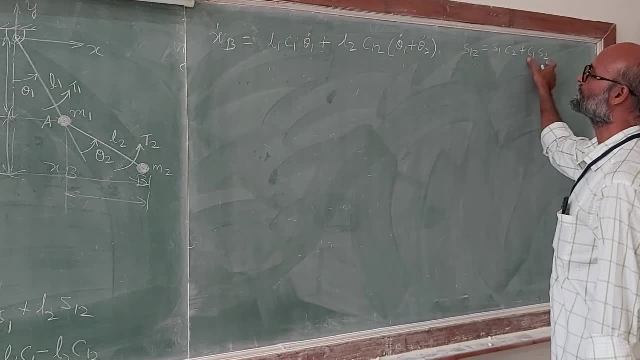 lid. you said the try to simply chop off y tu, but I am going to do it. c 1, y a dot, But this aberration is really he power. All right now, what we are going to do is demonstrate it like this. So we are going to divide it in half. So if we take this, lots but both. 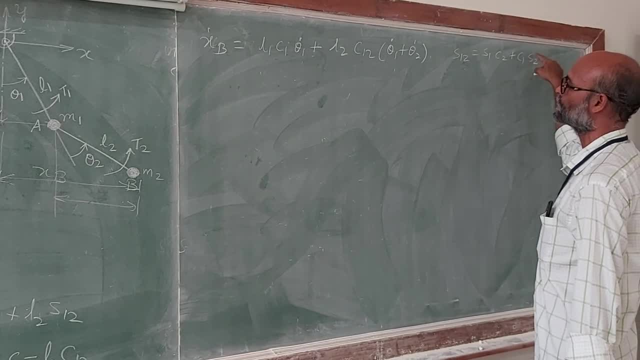 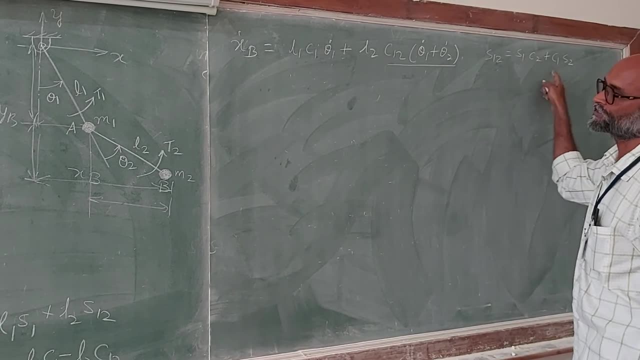 ways. do it So when we divide it h2. so if y and y is equals this one, If you choose, you have to differentiate using product rule. then you will get this term, whatever I have written here. So use this differentiation technique to get this x dot p. What about? 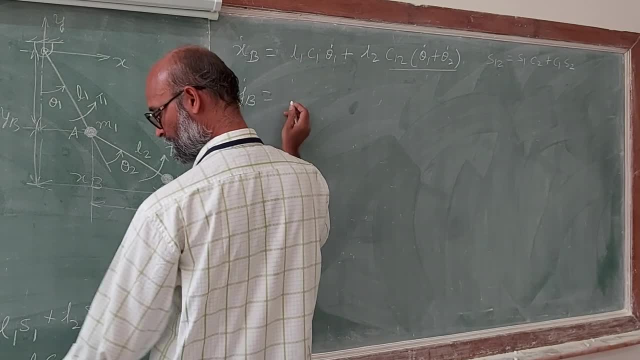 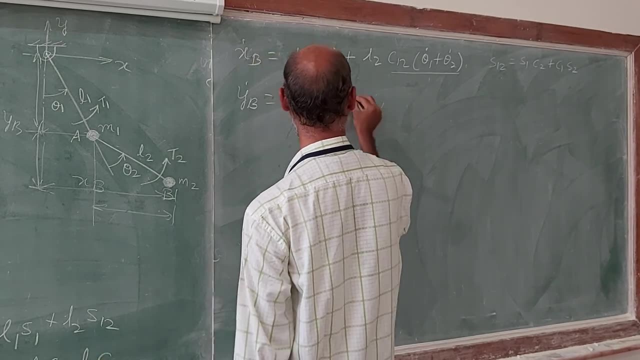 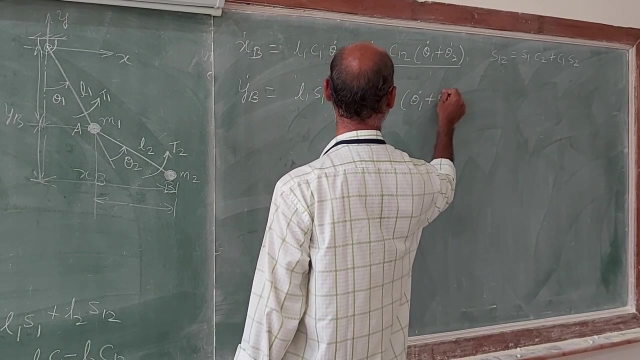 y dot p. On the same lines. this will be: it is minus. since it is already minus, this will become l 1, s 1, theta 1 dot. this becomes plus l 2, s 1, 2, theta 1 dot plus theta 2. 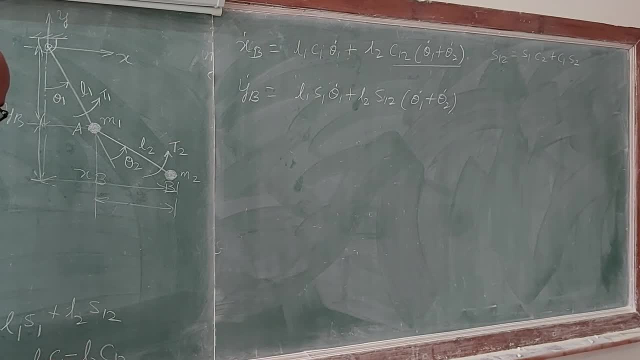 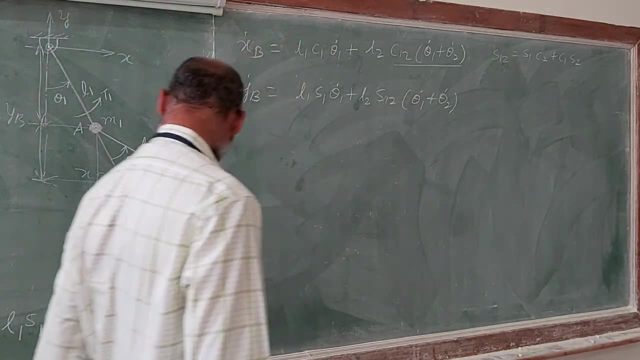 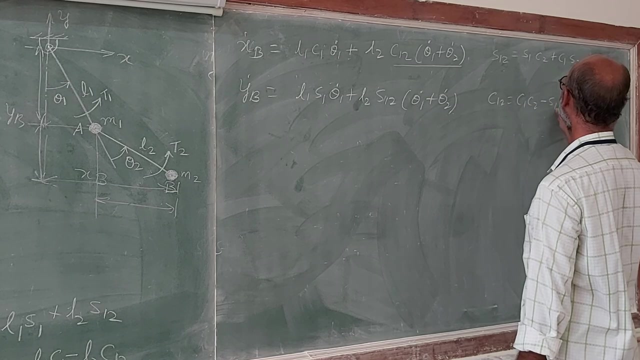 dot. So differentiation of this, this minus, vanishes, because this is c 1,. differentiation of c 1 is minus s 1 and theta 1 dot, So that minus vanishes. here Again, if you write: this is c 1, 2,, c 1, 2, what is c 1, 2?? c 1, 2 is c 1, c 2 minus s 1, c 1, c 2 minus s 1, this. 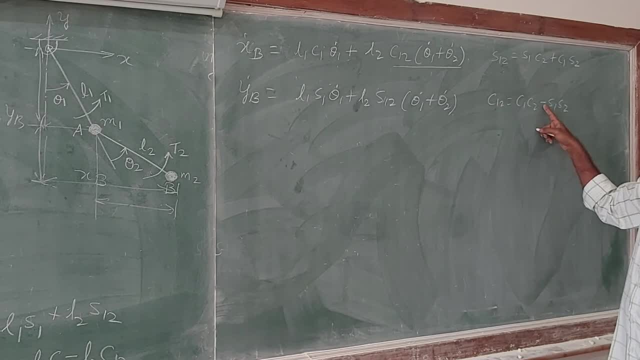 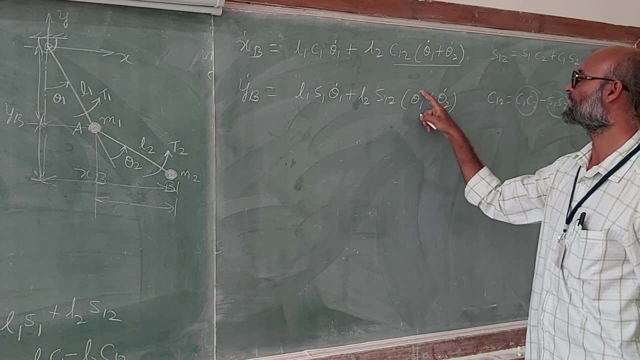 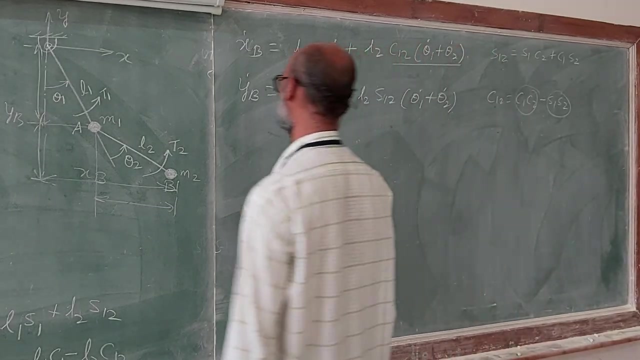 is? please note, it is cos a plus b, cos a plus b minus psi a, psi b. You differentiate this using each term of the product rule. you will end up with this: s 1 2, theta 1 dot plus theta 2 dot. So this is x 1 dot, y 1 dot. What is the velocity term? v square. 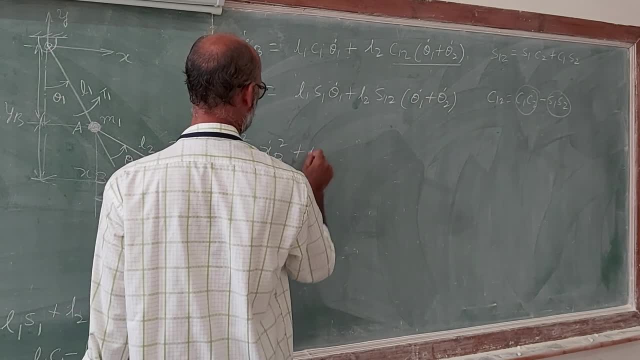 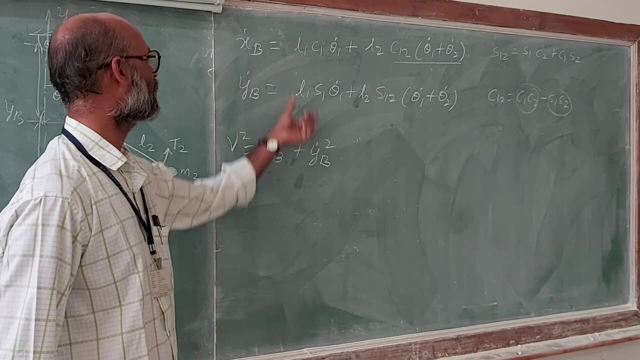 is x dot v square plus y dot v square. If you want velocity of this point, you need to square up these two and add these two. Let us do the exercise. So what is x dot square Square of this, whatever we have written? 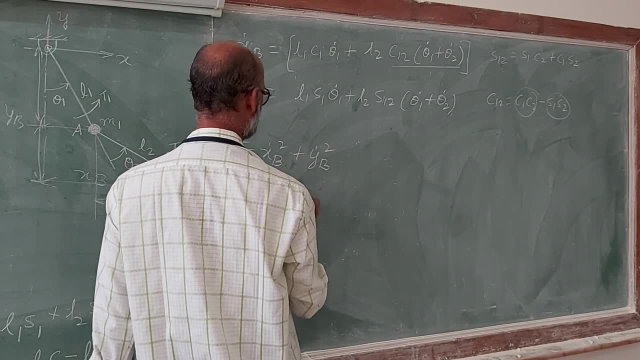 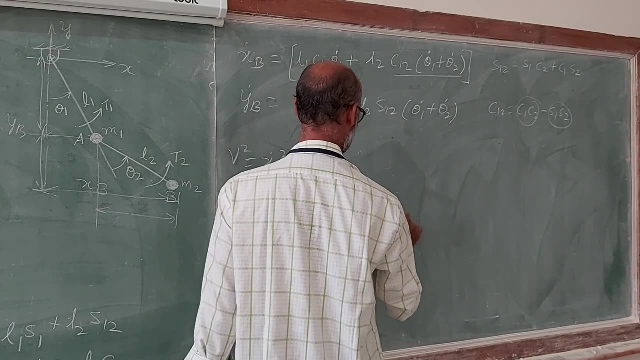 here square of this, that will be l 1 square c 1 square. theta 1 dot square plus l 2 square c 1, 2 square. theta 1 dot plus theta 2 dot. whole square. That is a square b square plus. 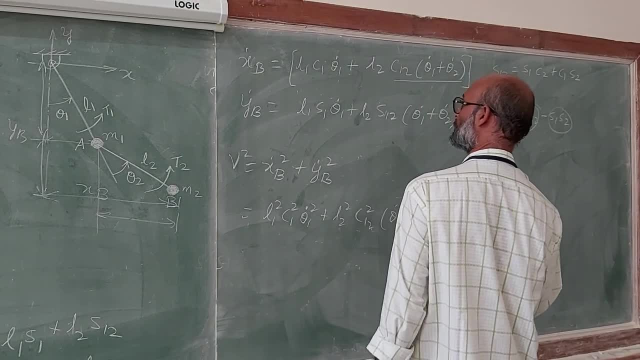 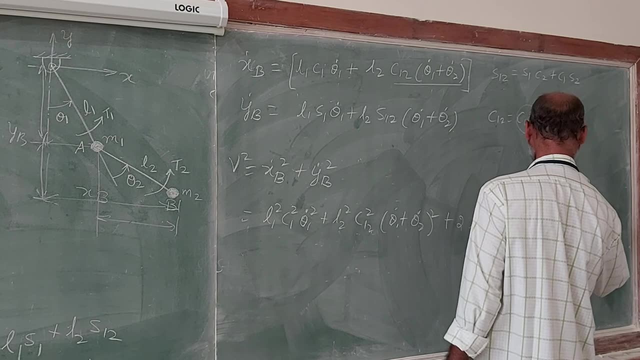 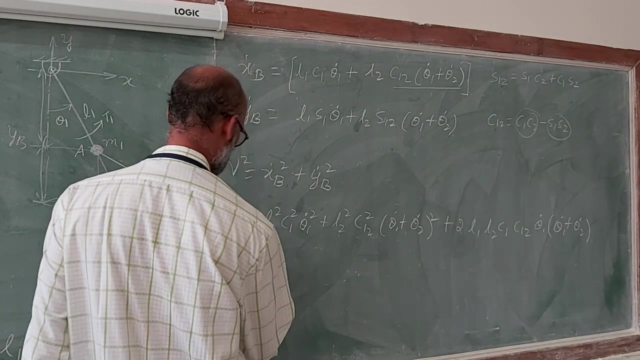 2 times l 1, l 2, c 1, c 1, 2.. So this is the square term of this x dot v equation. Whatever the square term of this plus this is only x p, now we are getting y dot v. the square of this term, This is: 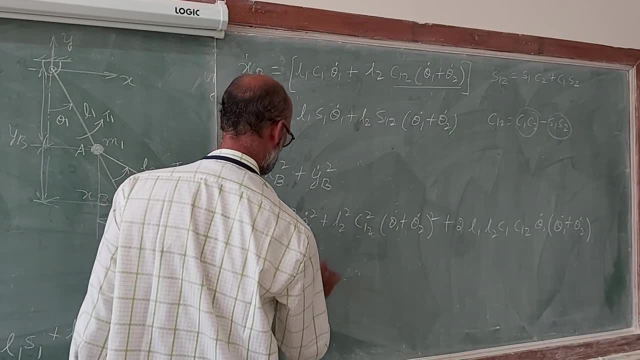 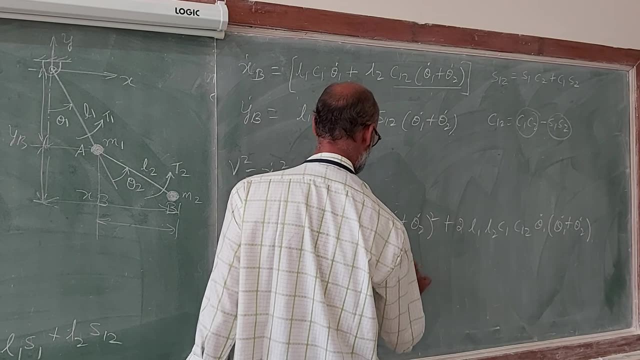 l 1 square s 1 square, theta 1 dot square plus l 2 square s 1, 2 square. and theta 1 dot plus theta 2 dot plus 2 times l 1 square. So this is the square term of this equation. 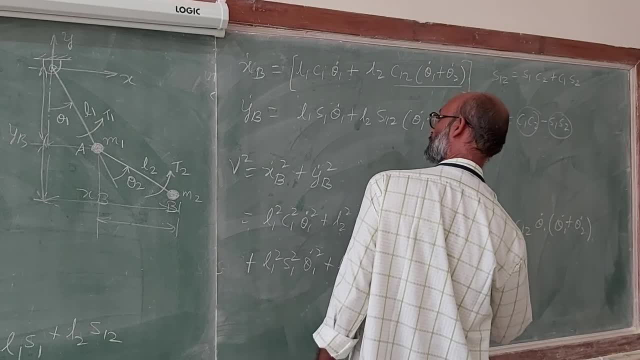 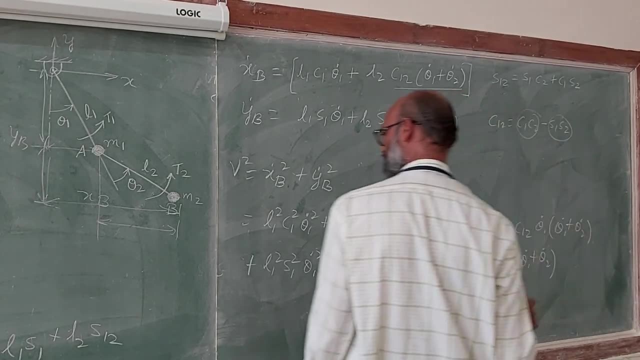 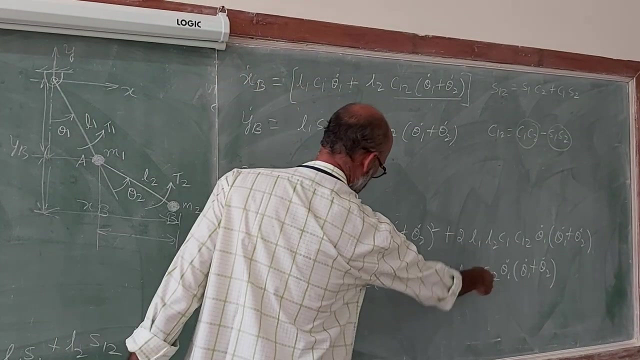 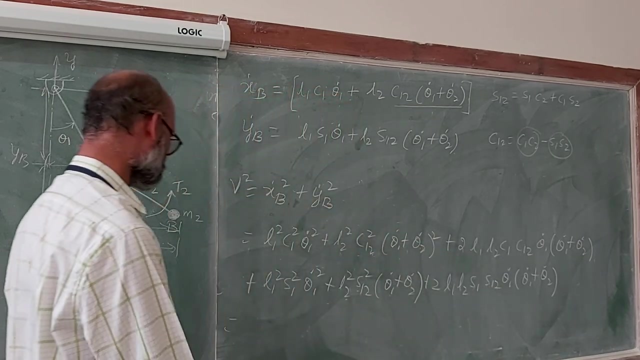 Now we can do two things: appeals. So this is your food square term. we will simplify this. We will look at this. We just add up these two terms. So this is this The 2nd. like what you see here, there is square for this: a square plus b square plus twice of. 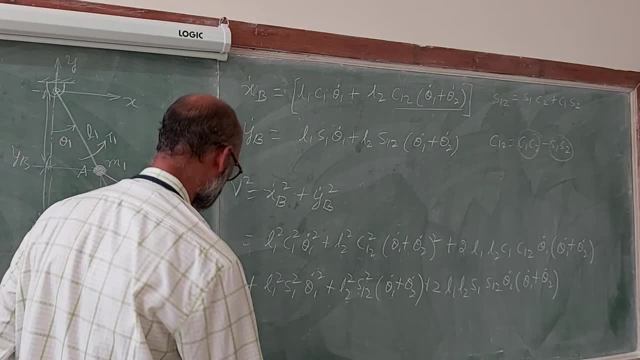 whatever i had written here. When you want to simplify this plus this, we can say: theta 1 dot square c 1 square, pri c 1 square. that is a square. So that will port. now we have square plus S 1 square. this will give you 1. so you get this as L 1 square, theta 1 naught. 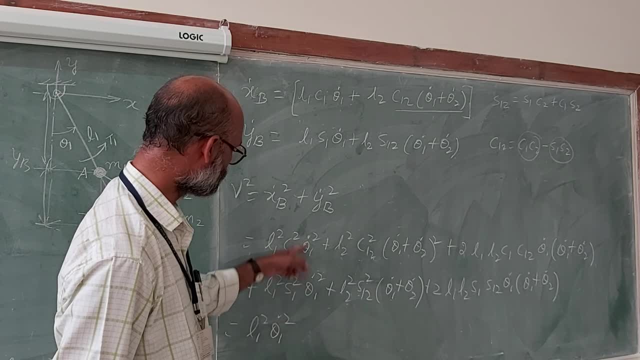 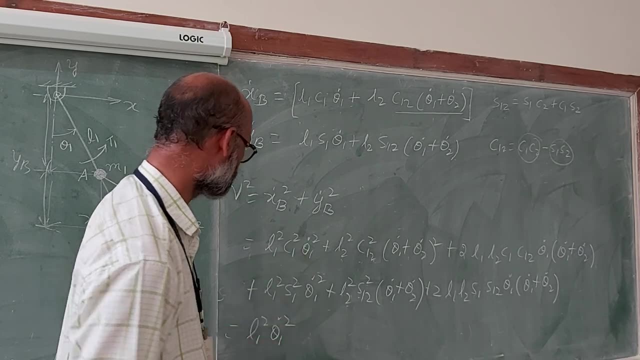 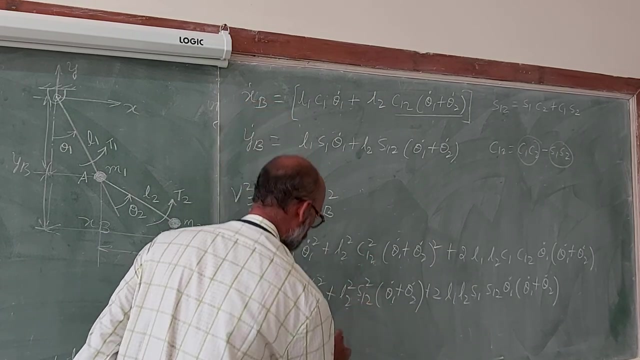 square. so I am adding up. when you add these two, since it is theta 1 naught square, you can add up. so C 1 square plus S 1 square, you get 1, so L 1 square and theta 1 square remains here. similarly, here you get this as L 2 square, C 1, 2 square plus S 1 square is again 1, so 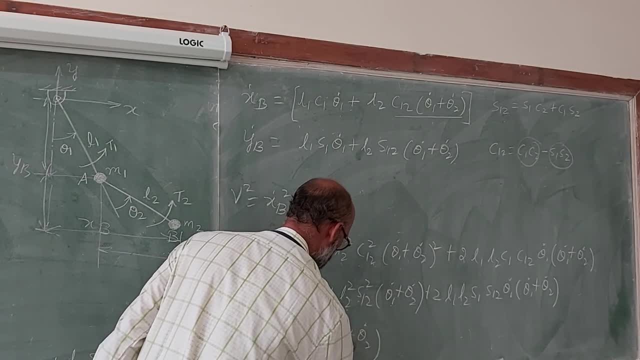 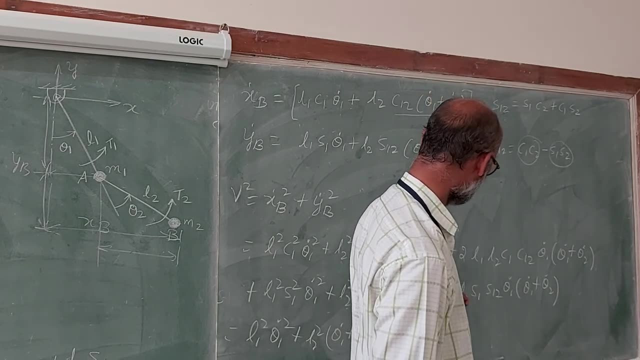 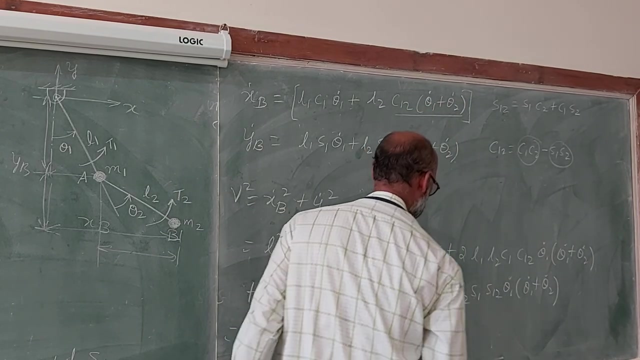 you get this as theta 1 naught plus theta 2 naught 4 square. that remains in these two terms and if you add up these two, please see 2 L 1, L 2 are common here. please note that plus 2 L 1, L 2 and this term is also common. I will leave it out theta 1 naught. 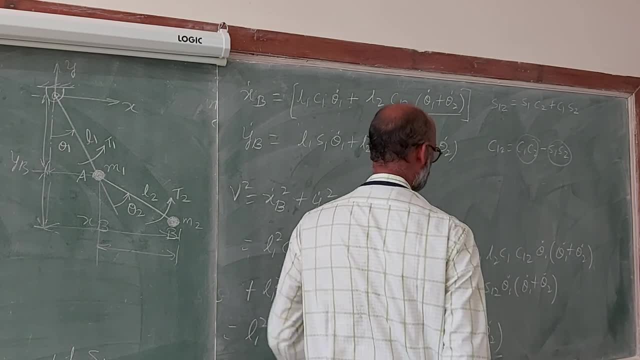 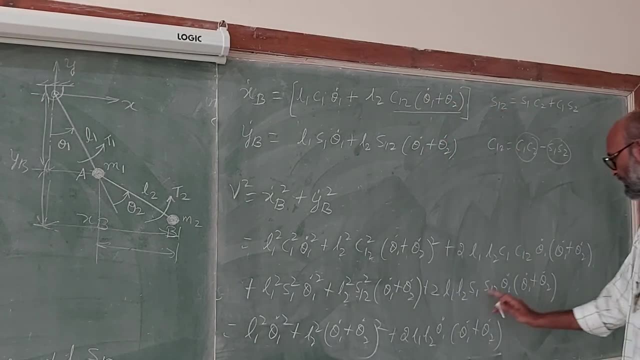 theta 1 naught plus theta 2 naught, you have addition of C 1, C 1, 2 plus S 1, S 1, 2. if you add up. what I mean to say is, if you look at here, you get C 1, C 1, 2 plus S 1, S 1, 2 you. 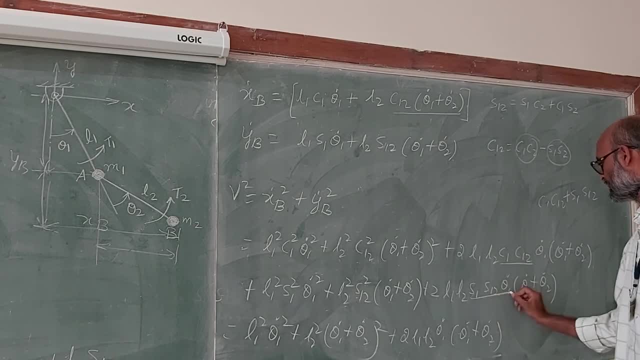 have addition of C 1, C 1, 2 plus S 1, S 1, 2 if you add up. what I mean to say is, if you look at here, you get C 1, C 1, 2 plus S 1, S 1, 2. that is the addition for these two terms. 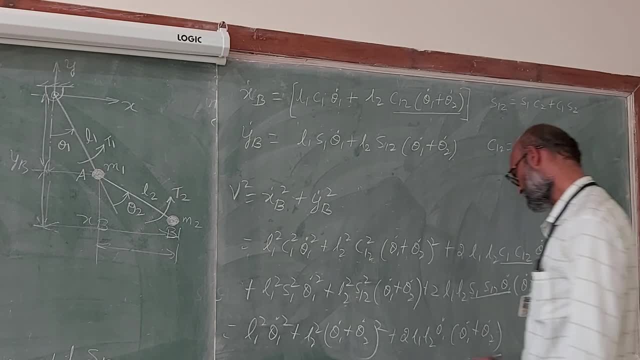 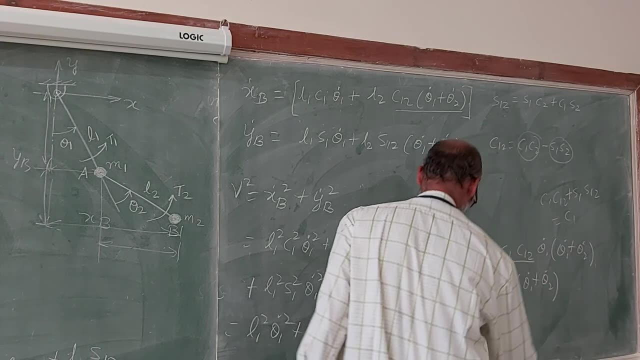 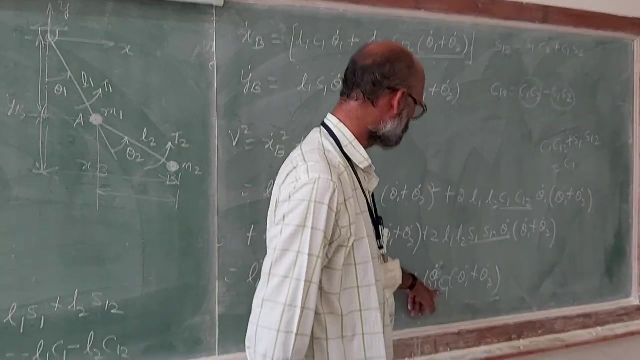 this comes to be C 1 if I, if my memory is right. I think it should be C 1. you can evaluate cross theta 1 and you have to evaluate these two equation and you will get this as C 1 and you will write it as C 1 here. please note: this is theta 1 naught. so how did we get this? 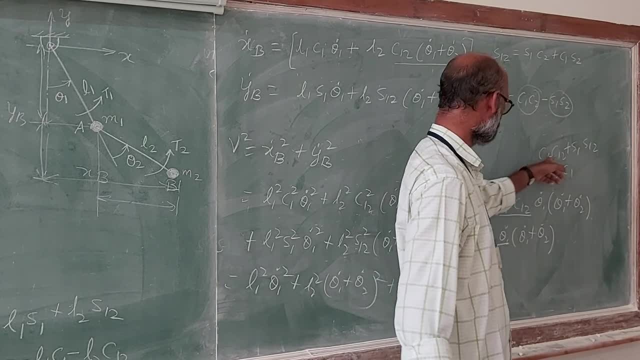 C 1. C 1 is because of this equation, addition of these two terms. okay, Thank you. Thank you.